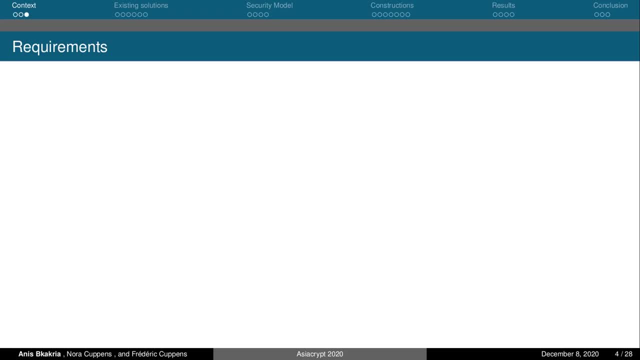 content inside the data. so in this work we are interested in a solution that is: first, security, where, in the sense that it should allow pattern matching on encrypted data, second market complaint, meaning that, except the pattern provider, detection patterns should be indistinguishable to all other involved parties. in addition, the pattern provided by the pattern matching service, 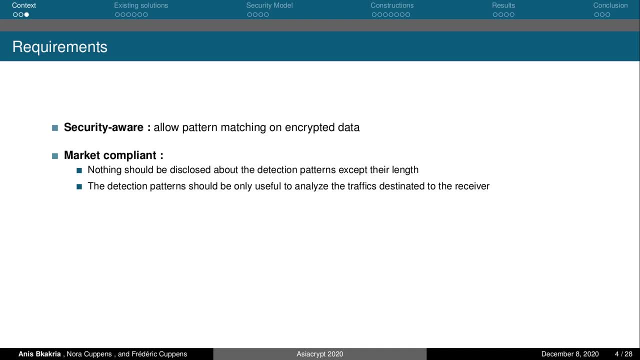 provider should be useless to analyze or the third-party encrypted data otherwise. Otherwise, the pattern matching service provider can create value by selling them to other security service providers. The solution should also be privacy-preserving, meaning that, except the sender and the receiver, 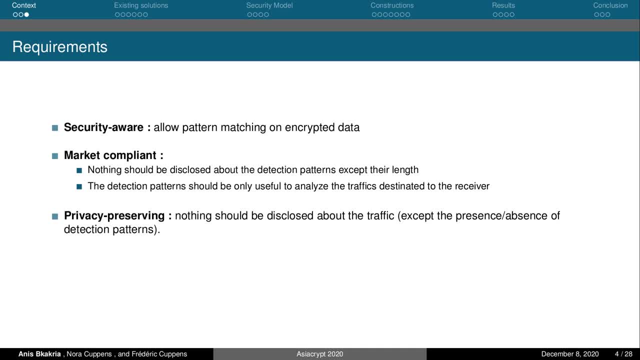 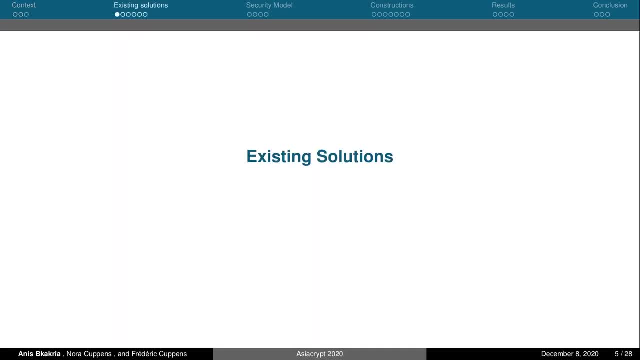 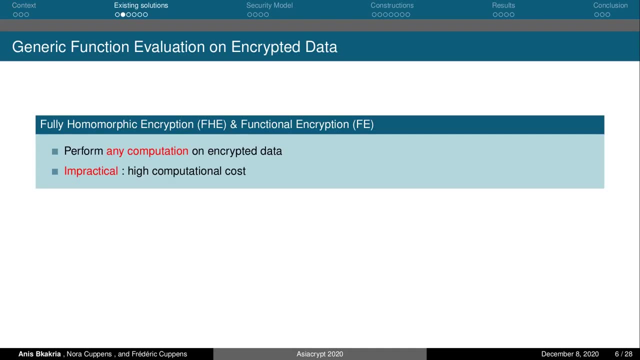 encrypted data should be indistinguishable to all other parties. Finally, the solution should be more practical compared to existing ones. Multiple techniques can be used to perform pattern matching on encrypted data. Generic solutions, such as fully homomorphic encryption and functional encryption, can be. 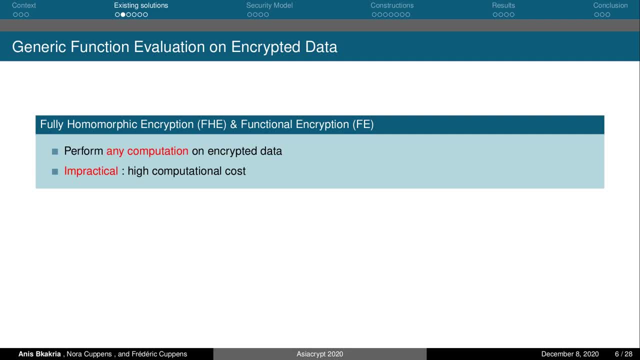 used to perform pattern matching. Still, these techniques are unpractical because of the high cost of the computation they require. Multiparty computation can be also used to perform interactive computation on encrypted data. However, performing pattern matching using multiparty computation requires a high number. 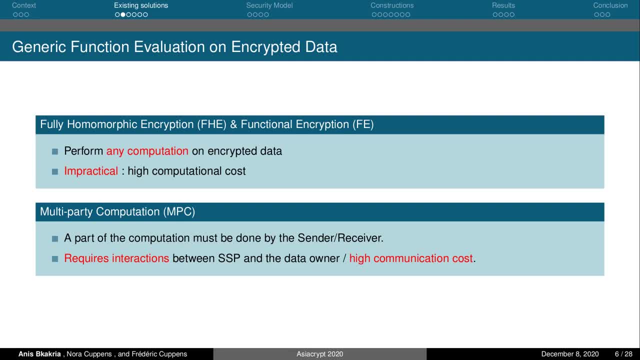 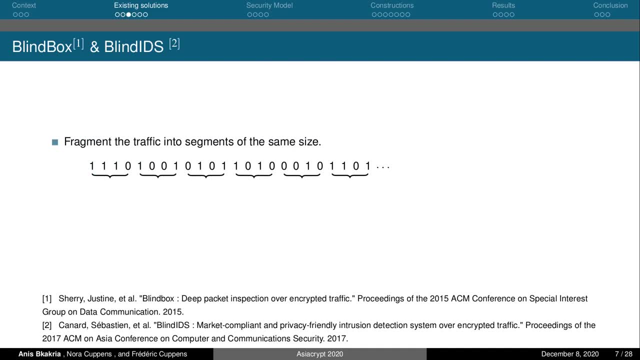 of interactions That is, in the worst case, linear to the size of the data, which results in very high communication costs. Blind Box and Blind IDS are two solutions that have been proposed for signature-based introduction detection on encrypted data. The idea consists of splitting the data to be encrypted into fragments of the same size. 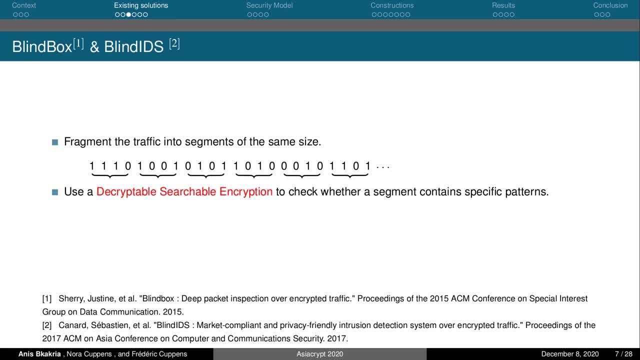 Then they used a construction called decryptable- searchable encryption- to check the presence of attack signatures in these fragments. Unfortunately, Blind Box and Blind IDS are useful only if all patterns have the same size. This, however, is not the case in practice. 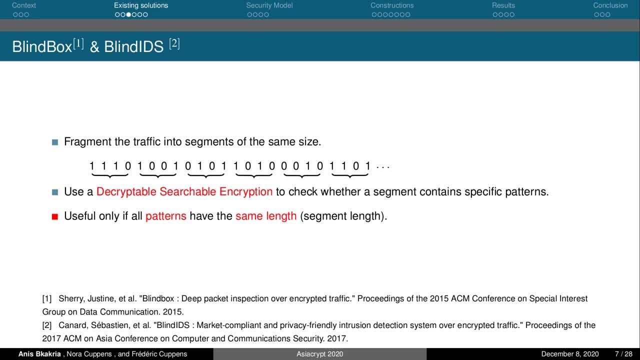 For example, the detection patterns used by the Snort tool have around 900 different sizes. In addition, these solutions may cause false negatives since, even if the patterns are all of the same size, they cannot be detected if they straddle two fragments. 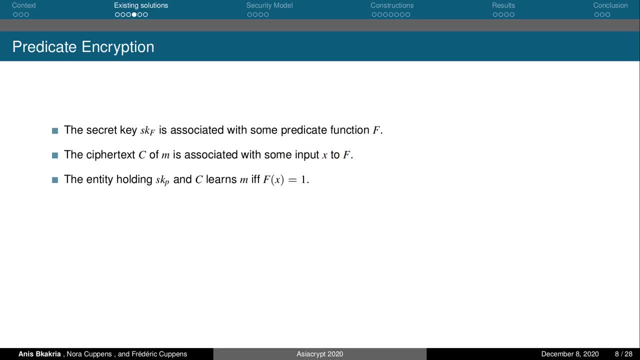 Predicate. Encryption can be used to detect the presence of attack signatures in the same size. The encryption can be also adapted to allow pattern matching on encrypted data At a very high level. the idea consists of considering each symbol in a detection pattern as an attribute of a predicate. 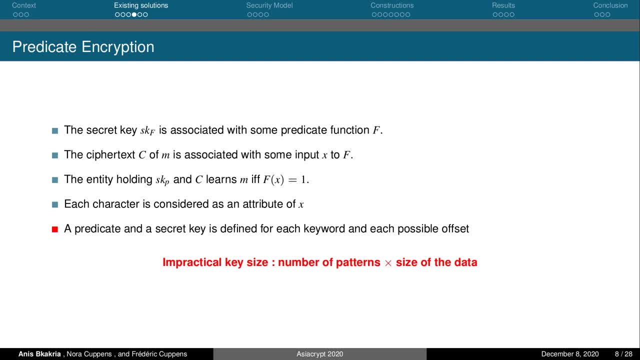 Then, to allow finding the patterns anywhere in the encrypted data, a predicate will be assigned to each pattern and to each possible position in the data to be analyzed. So we will end up requiring a secret key of the size linear to the size of the traffic. 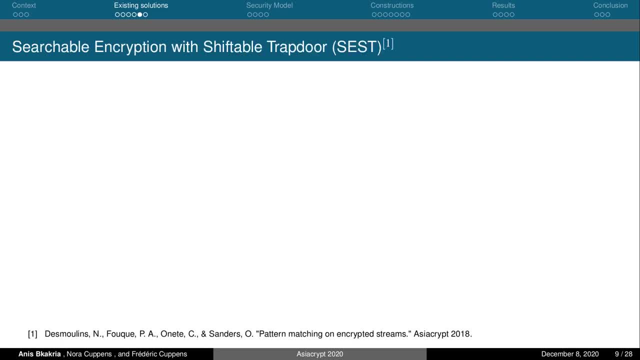 to be analyzed. Searchable Encryption and Searchable Encryption can be also adapted to allow pattern matching on encrypted data. Searchable encryption with Siftable Trapdoor has turned out to be the most interesting solution for pattern matching on encrypted data. It is based on an asymmetric construction that supports searching for arbitrary patterns. 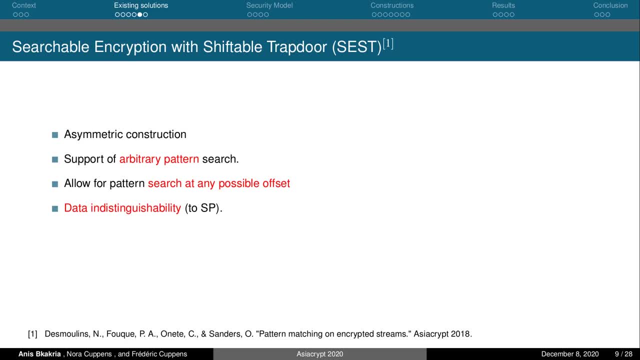 at any offset of the data, while ensuring traffic and distinguishability to the pattern matching service provider. Still, this solution cannot fully protect the detection patterns. In addition, it requires a public key of the size linear to the size of the traffic to be analyzed. 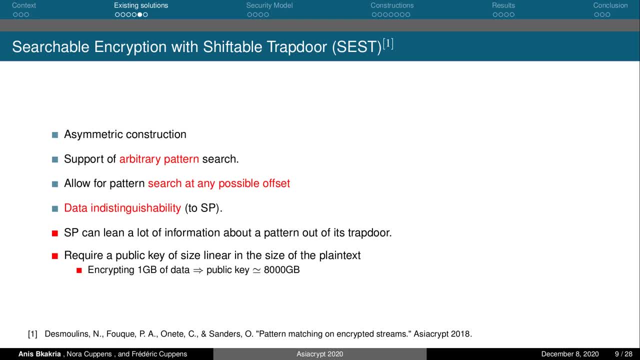 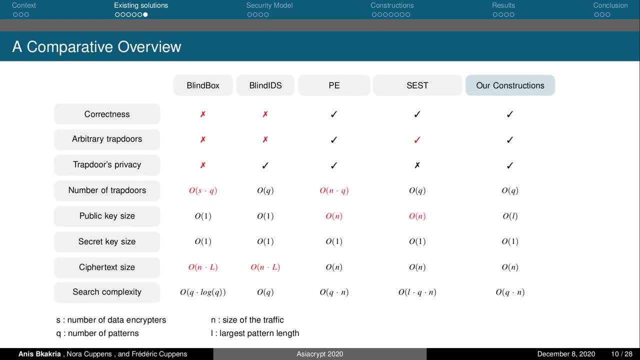 So concretely, if we want to exchange one gigabyte of data, we will need a public key of eight terabytes. Compared to the previous solutions, our scheme is the first that allow correct arbitrary pattern matching and ensure both data and pattern privacy without requiring a very large 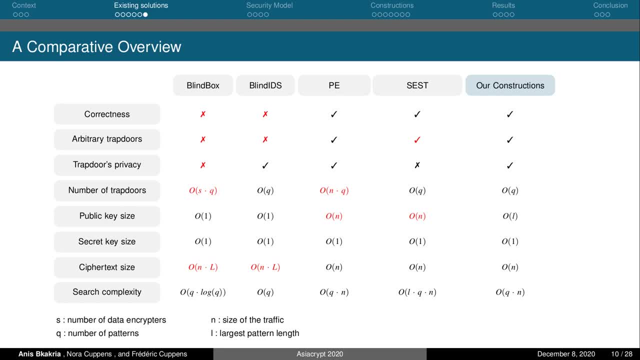 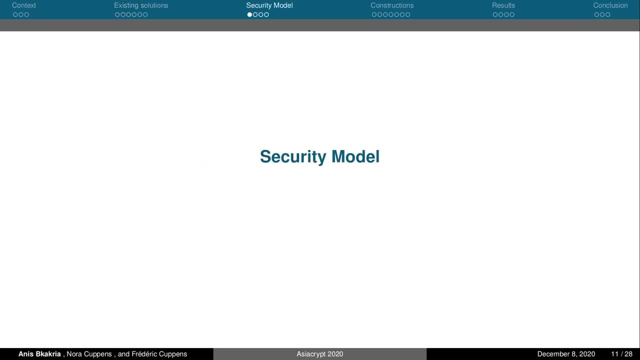 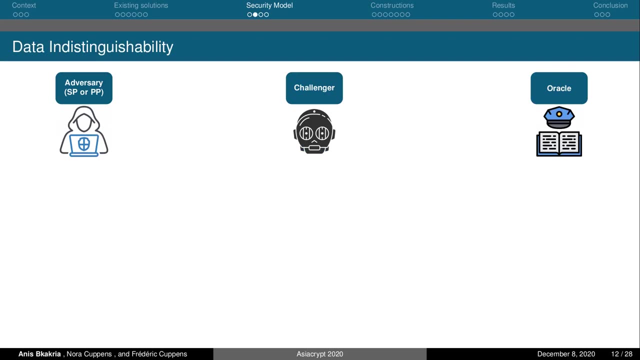 number of trapdoors, which is the case of predicate- and create Corruption or very large keys, which is the case of SEST. So let us move forward and see the security model we consider. Data and distinguishability requires that. it's not feasible for the service provider. 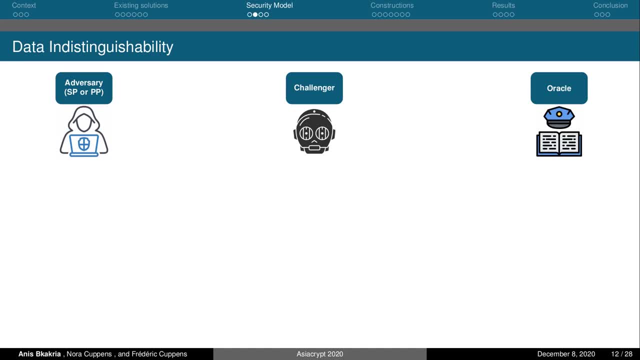 or the pattern provider to learn any information about the traffic other than the presence or the absence of specific patterns. We model this property as a game between an Adversary and the challenger, So the adversary starts by getting the encryption and trapdoor generation key. 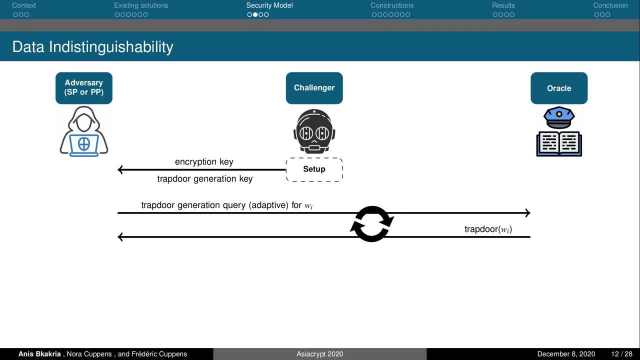 Then he is allowed to adaptively perform a polynomial number of trapdoor generation queries for patterns of his choice. Once he decides that this query phase is over, the adversary chooses two traffic that do not contain the previously created patterns and send them to the challenger, who chooses. 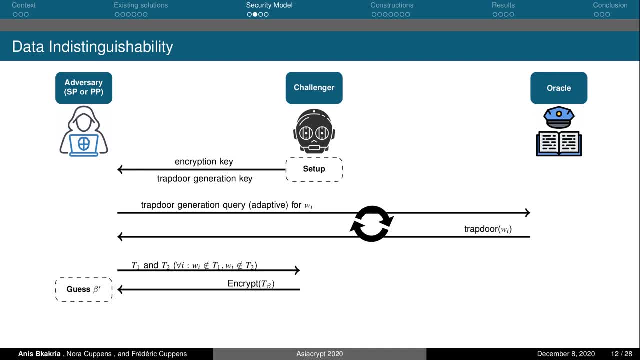 one of them. He encrypts it and sends it back to the adversary. The adversary wins the game if he manages to figure out the traffic that has been encrypted by the challenger. In addition, we consider the pattern and distinguishability property, meaning that it's not feasible. 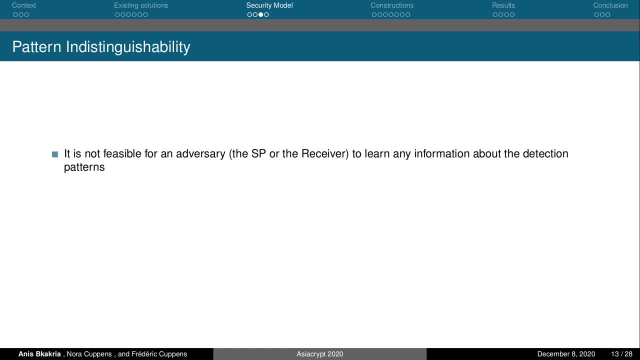 for the SP or the receiver to learn any information about the detection patterns. We will consider the case of a public key encryption in which the adversary can encrypt any traffic of his choice. This allows him to mount a brute force attack on the detection patterns. 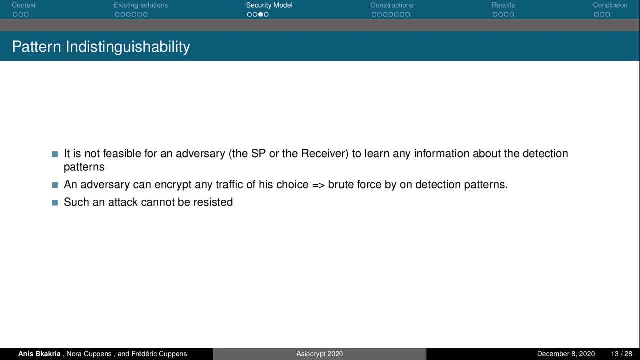 Unfortunately, in this case, no pattern matching based solution over either plain text or public key encryption ciphertext can resist such an attack. Therefore, this brute force attack should not be considered in our security model. One solution to dismiss this type of attack is to consider an adversary having high mean. 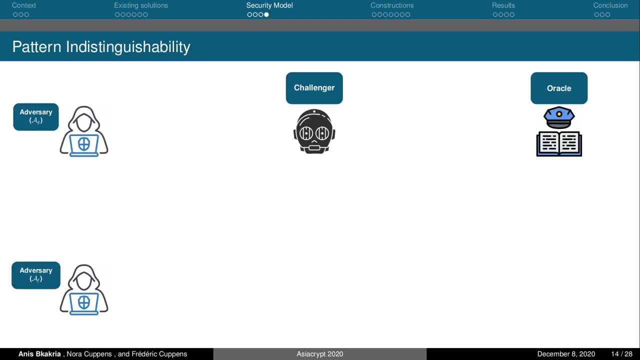 entropy, Which is usually modeled. This is modeled using two non-colluding entities, AF and AG. As usual, the entity AG of the adversary starts by getting the encryption and the trapdoor generation keys and adaptively perform a polynomial number of trapdoor generation queries for 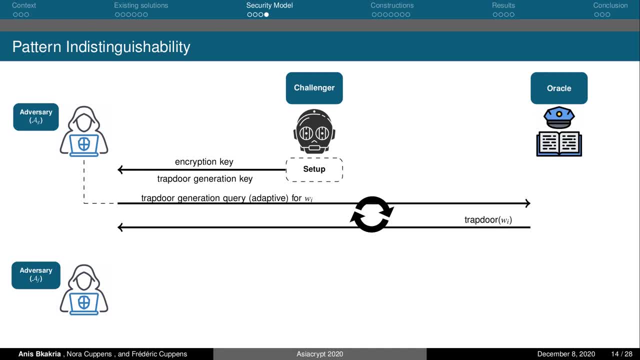 patterns of his choice. Then the same entity chooses two trapdoors that were not used in the previous trapdoor generation queries and sends them to the challenger who chooses one. This is called a trapdoor generation query. The trapdoor generation query issues a trapdoor for the chosen pattern and sends the trapdoor. 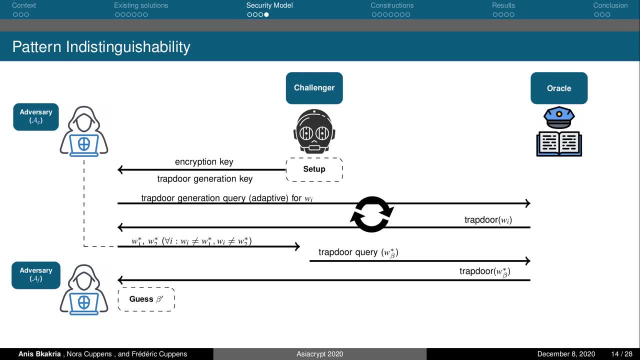 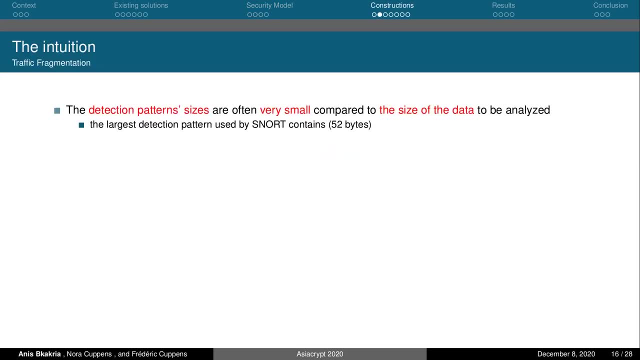 to the entity AF of the adversary. The adversary wins the game if the entity AF manages to figure out the pattern that has been chosen by the challenger. All right, let's see now our construction more in details. The intuition behind our solution relies on the fact that the sizes of the attack's pattern 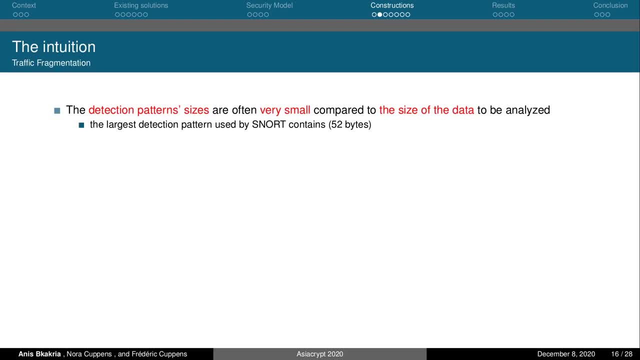 are very often minuscule. For example, the largest detection pattern used by the snort tool contains only 52 bytes, So the idea is then to fragment the data into a set of small segments of the same size and encrypt each of those segments separately. 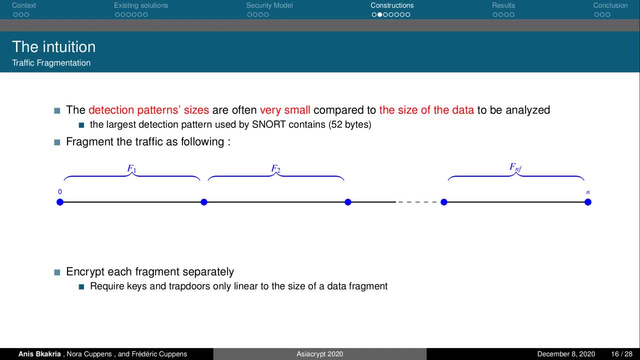 Now, instead of requiring keys and trapdoors of size linear to the size of the data, which is the case of the most existing solutions, This fragmentation technique will enable us to construct a scheme that requires keys and trapdoors of the size only linear to the size of the data fragment. 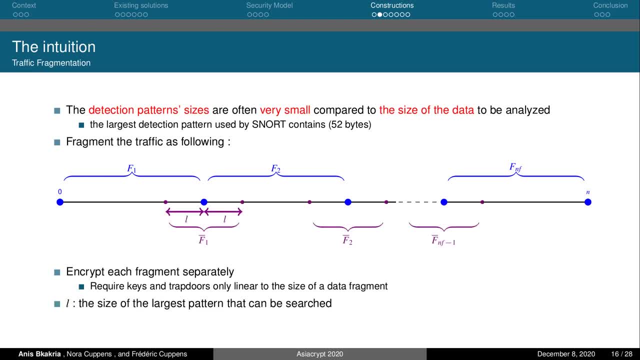 And to allow detecting the patterns that may straddle two fragments for each two neighboring fragments, we build a third one which will be composed of the last L elements of the left side fragment and the first L element of the right side, one with L representing. 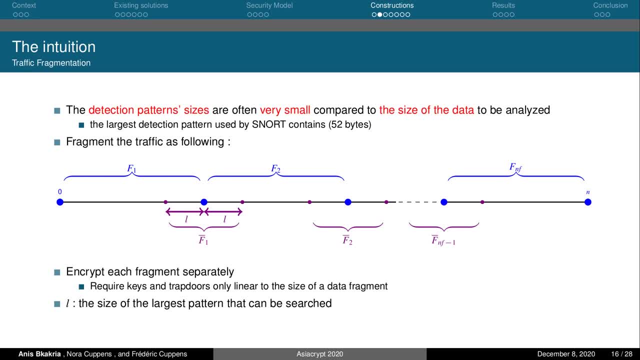 the largest pattern size that can be searched on the left side of the data fragment. This will allow us to construct a scheme that requires keys and trapdoors of the size only linear to the size of the data fragment. Concretely, if we want to be able to search all detection patterns that are used by the 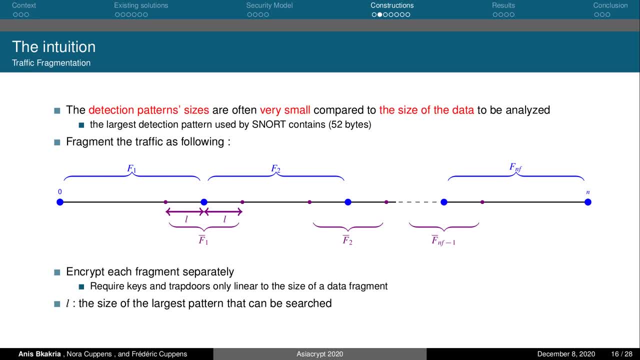 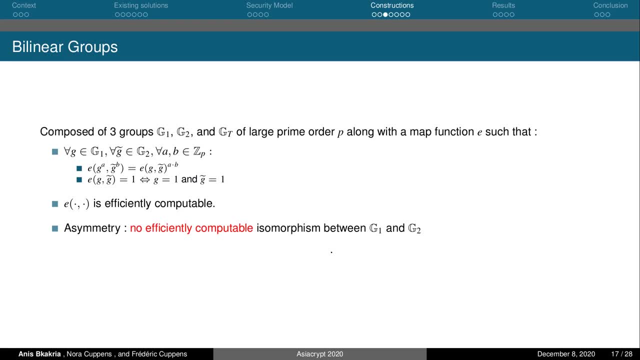 snort tool L should be greater or equal to 52 bytes. Our construction is based on asymmetric linear groups. Roughly speaking, we consider three cyclic groups- G1, G2 and Gt- of a large prime order P and an efficiently computable mapping function, E that maps two elements of G1 and G2 to an. element of Gt in social. well, The first one is a function called the G1 function. The second one is a function called the G2 function. The third one is a function called the G2 function. The fourth one is a function called the G2 function. 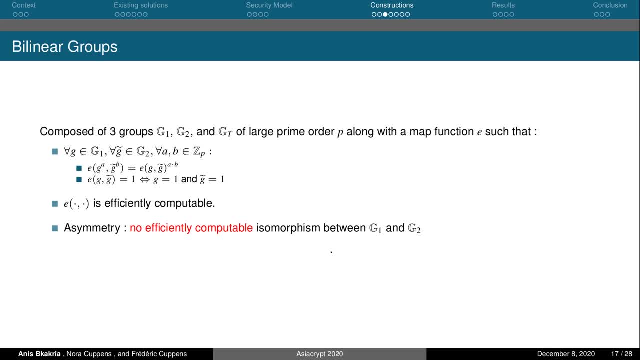 The fifth one is a function called the G2 function. The sixth one is a function called the G2 function. It's also called the G2 function. In summing up the project as a type of a master, true representation, We can. seventh, the 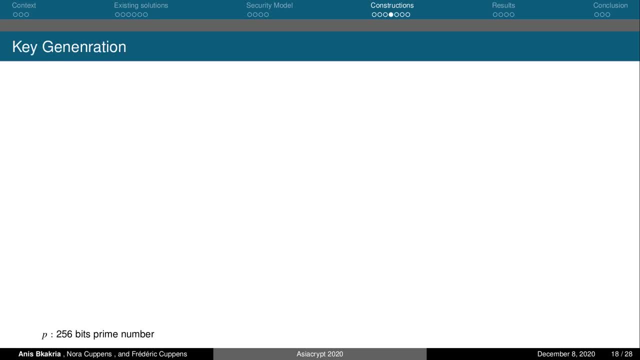 pressure of double split. Let's have a look at a example of such aности representation: A four dimensional Lucas's vectors e scholars. Some of them will be used to encode the different symbols used to represent the data. If we consider the data as a bit string, we will encode each. 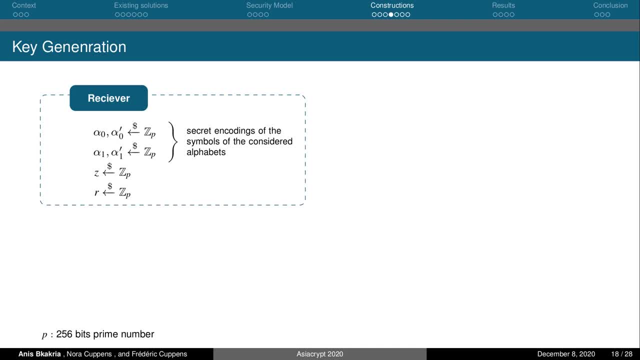 of the bits 0 and 1 using two random scholars, alpha and alpha prime. These random scholars will represent the secret key of our construction. Using this secret key, the receiver generates a public key composed of a set of couples of elements of the cyclic group G1.. The left side elements of these couples can: 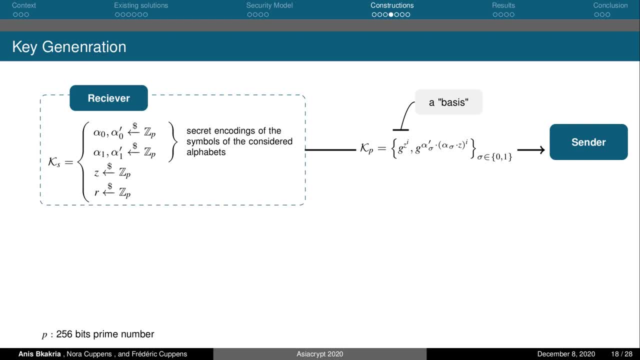 be seen as a public basis, where I represents the different offsets in the data fragment, while the right side elements represent the projection of the different symbols of the alphabet used to represent the data on the basis. Finally, the receiver computes the trapdoor generation key KT and sends it. 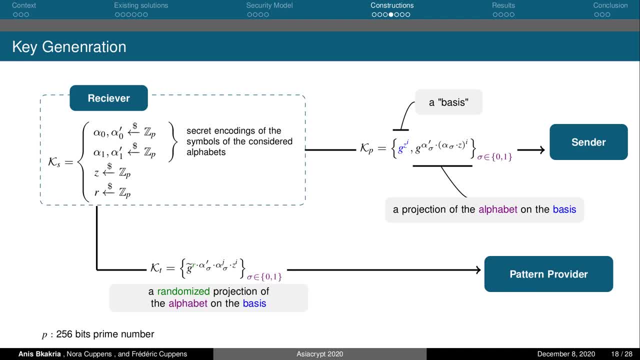 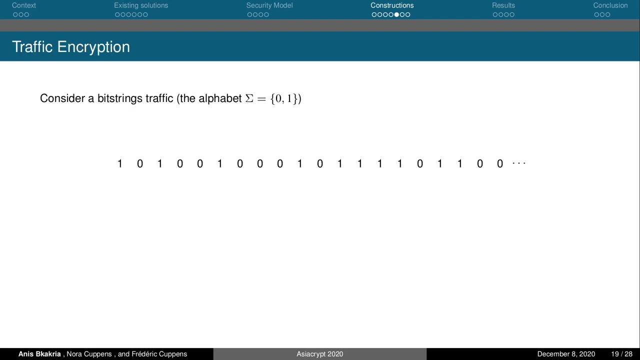 to the pattern provider. The elements of KT are actually randomized projections of the alphabet symbols on the basis. The randomization here is used to prevent the pattern provider from using the elements of the key KT to learn information about the encrypted traffic. To encrypt the traffic, the sender starts by generating for each fragment a large 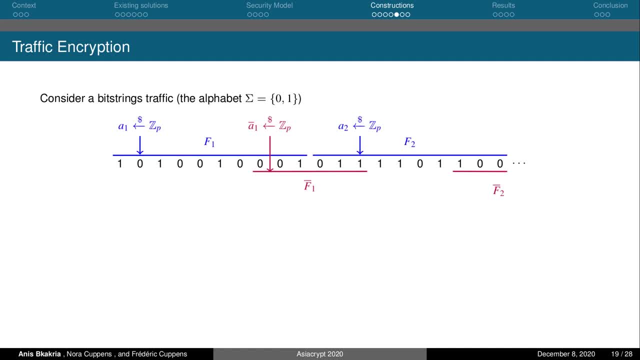 random scalar that will be used to randomize the encryption of each data fragment. This allows to prevent frequency attacks on the encrypted data. Then each symbol of the data will be encrypted separately. For that, the sender encodes each symbol into two elements of the group G1.. These elements are: 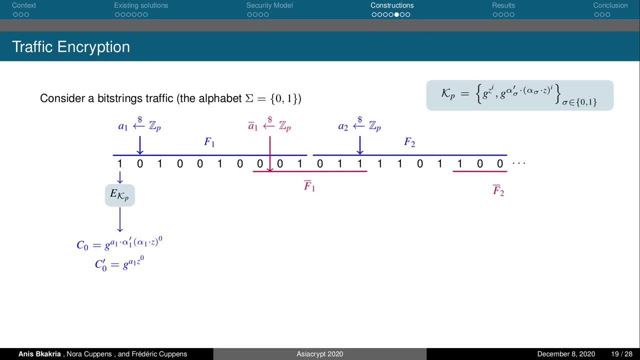 retrieved from the public key, where I represents the position of the symbol inside the fragment and Sigma represents the symbol to be encrypted. Then the two elements are randomized using this color a1 and we do the same for encrypting other bits. for bits that belongs to two data fragments, they will be encrypted. 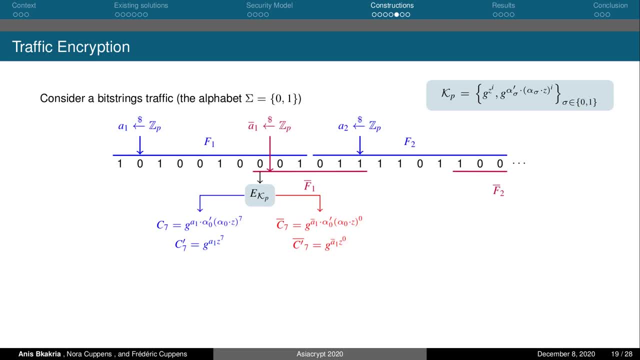 into four elements of g1, each couple of elements representing the encryption of the bit regarding its position in the corresponding data fragment. so the elements colored in blue represent the encryption of the bit regarding its position in the fragment f1, while the elements in red represent the encryption. 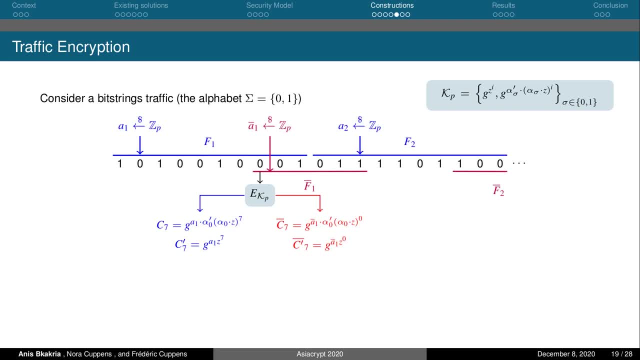 of the bit regarding its position in the fragment f1 over lined. so let's move now to see how the trapdoors will be generated by the pattern provider. let us suppose that we want to generate a trapdoor for the binary pattern 0 1- 0 and that the following scale represents the different offsets in a: 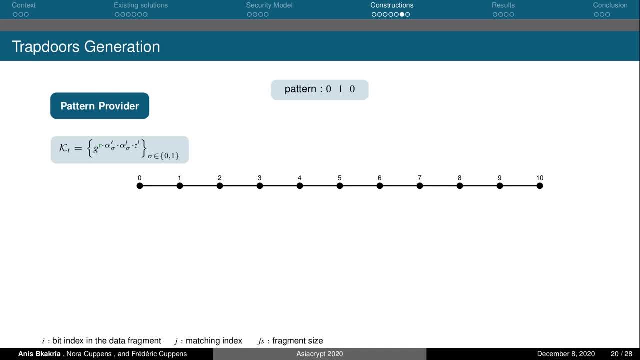 data fragment using the key KT. for each possible offset, the pattern provider will compute two elements of the group G2 as following: he will get three elements from KT, such that Sigma is the value of the bit of the pattern, I is offset of the symbol in the data fragment and G is offset of the pattern. 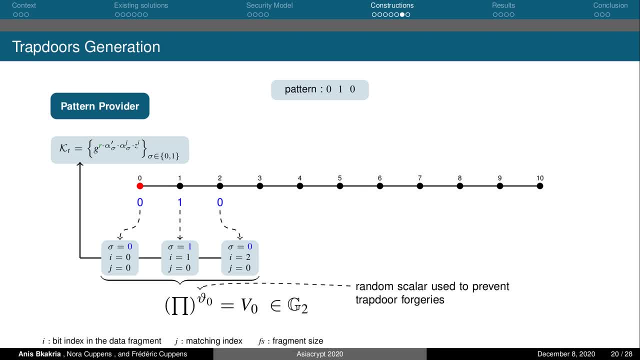 in the data fragment, the re-thrive. three elements are then aggregated and randomized to prevent trapdoor forgeries. the computed values v0 and the random value for Teta 0 are then added to the trapdoor as the elements allowing to search the pattern. 0, 1, 0 on the first position of a data. 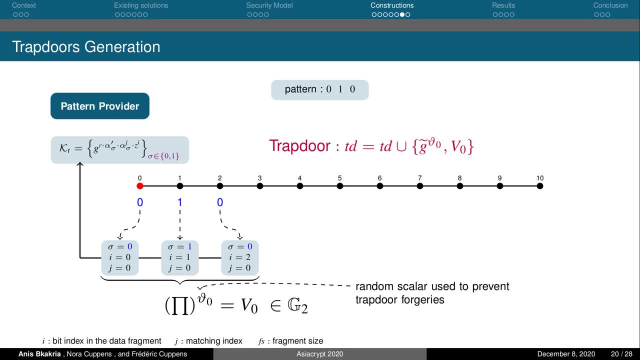 fragment. we repeat the same steps to compute and add to the trapdoor in the data fragment. We repeat the same steps to compute and add to the trapdoor in the data fragment door the elements of G2 that will be used to check the presence of the 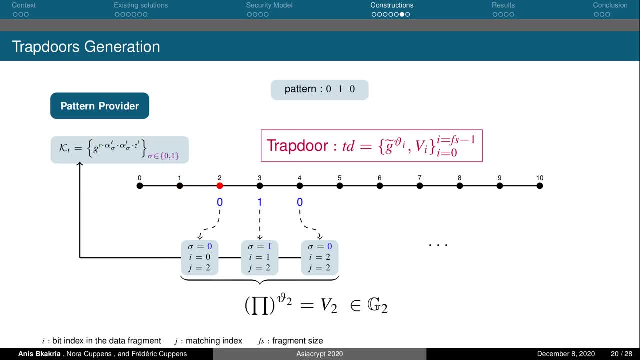 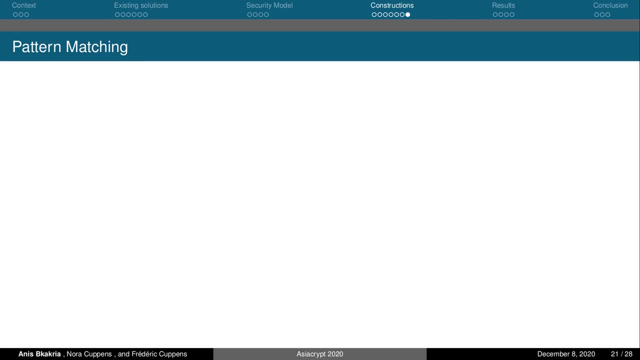 pattern at every possible position of a data fragment. at the end, the trapdoor will contain two times the number of symbols in a data fragment. elements of G2. all right now we have all the ingredients to understand how the pattern matching is performed by the service provider. let us suppose that we have the 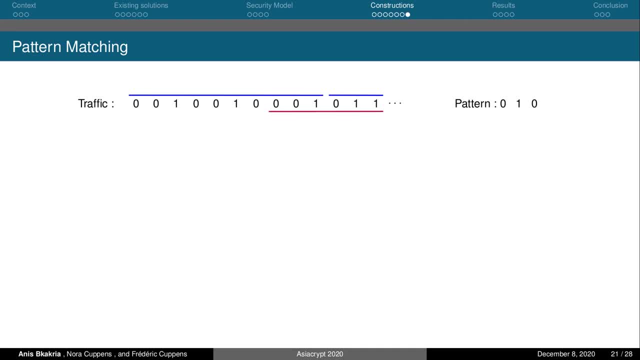 following binary traffic and the service provider want to look for the pattern 0, 1, 0. so for that he will check the presence of the pattern in all offsets, starting from the offset 0. so the service provider will get the encryption of the first three symbols of the traffic, together with the elements of the 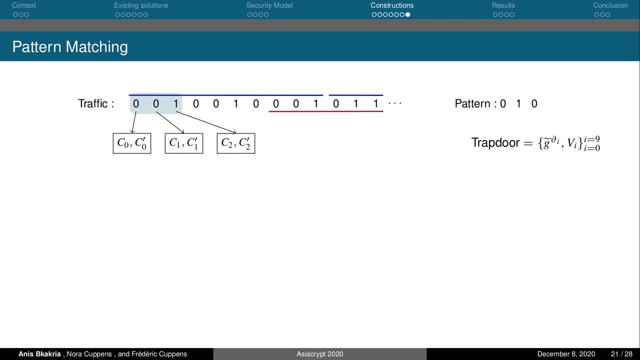 pattern trapdoor V0 and G2 and VAR theta 0 that allow to check the presence of the pattern at of F set 0. then he computes the pairing of the product of C 1, C 2 and C 3 and G tile to: 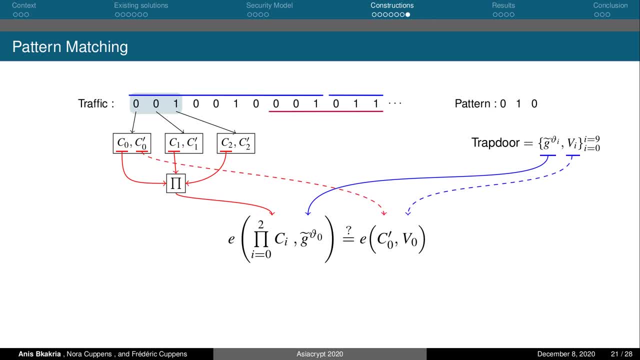 the power of VAR theta 0 and check if the result is equal to the pairing of C prime 0 V 0. if the equation does not hold, which is the case in our example, the service provider did use that the pattern is not. presence in the offset 0. 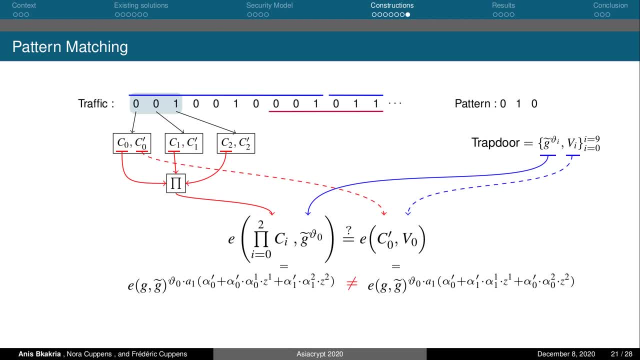 with overhelming probability. Otherwise, if the equation holds, which for example is the case for the offset 1, then the service provider will be sure that the pattern exists in the checked offset. I want to emphasize here that, regardless the results of this equation, the values of the two 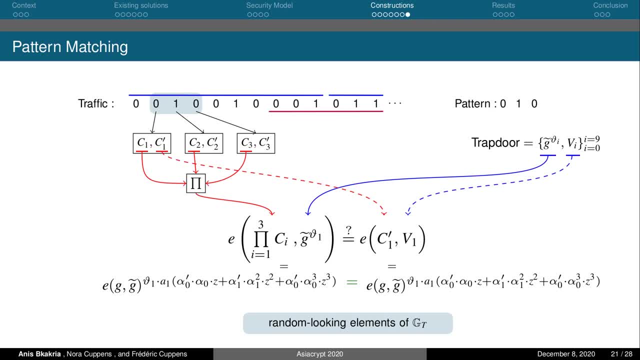 sides of the equation will be random looking elements of gt which will be useless to the service provider for learning any additional information about the plaintext or the searched pattern. Now let's jump to an offset in which the pattern straddles two blue fragments. The idea here: 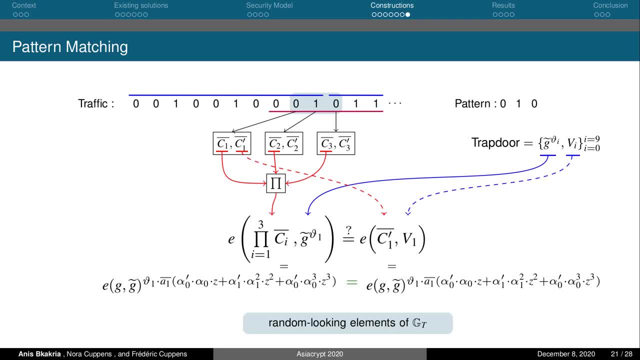 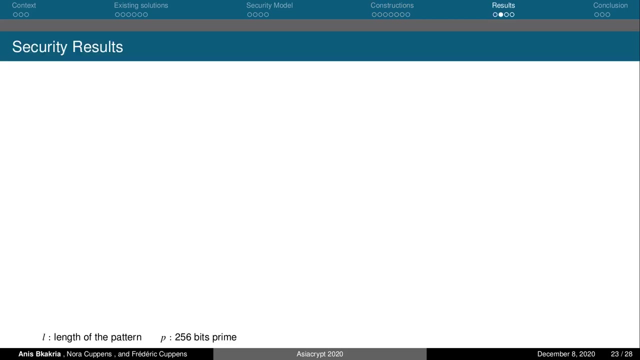 is to check the presence of the pattern in the red fragments. So use the encrypted elements regarding the offset of the pattern inside the red fragment and we check again the equality of the two pairings. All right, let's move on now to see the obtained results. From the security point of view, our 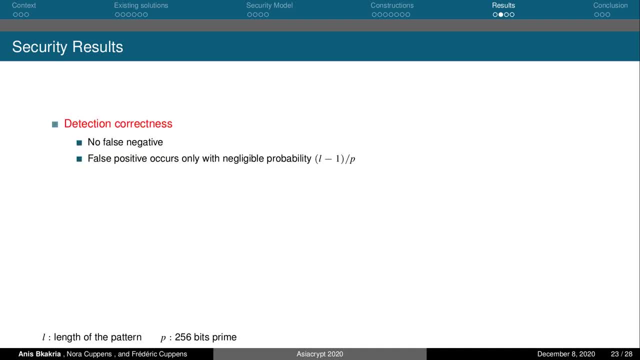 constriction provides correct detection of arbitrary patterns. Correctness here means that our constriction returns no false negative and that the probability that it returns a false positive is negligible. Our constriction ensures traffic and distinguishability to both the pattern and the service provider. This means that these two entities will learn nothing about the encrypted. 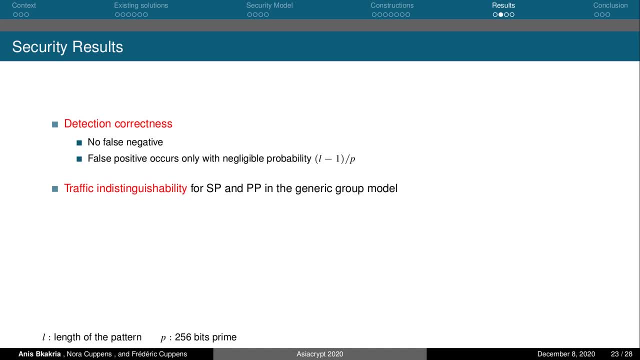 data, except the presence or the absence of the detection patterns. In addition, our constriction ensures pattern and distinguishability to both the service provider and the receiver, and this for detection patterns of high mean entropy. For evaluation results, our constriction requires a secret key composed of a secret key and a secret key composed of a secret key and a secret key. The 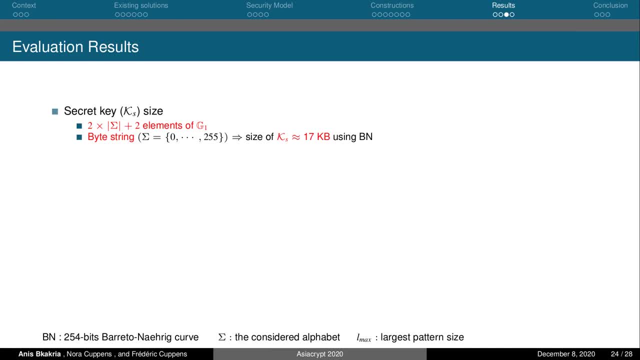 secret key is composed of two times the size of the considered alphabet, plus two elements of g1. So concretely, if we work with byte strings, the size of ks will be around 17 kilobytes. when using the bn elliptic curve, The public key is composed of four times the size of the. 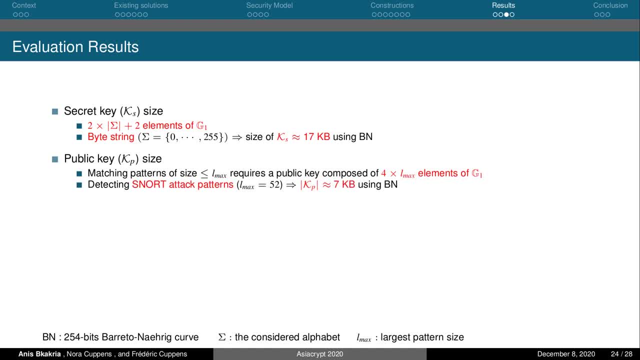 largest pattern that should be matched Concretely. if we want to match the detection patterns used by the snore tool, we will require a public key of only seven kilobytes. In addition, our constriction requires a trapdoor generation key composed of two times the square. 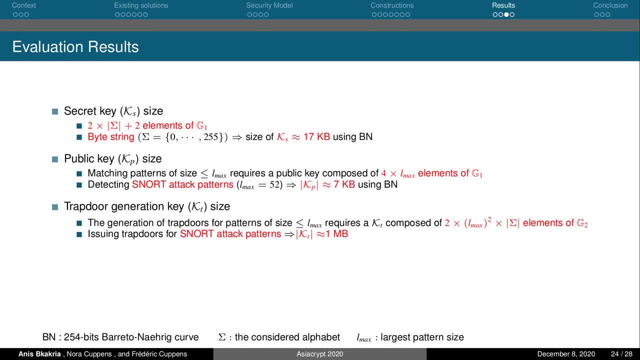 of the largest pattern size multiplied by the size of the considered alphabet elements of the group sheet 2.. Concretely, issuing trapdoors for snore detection patterns requires a key kt of a size around 1 megabytes. Moreover, our constriction requires trapdoors that are composed of two times. 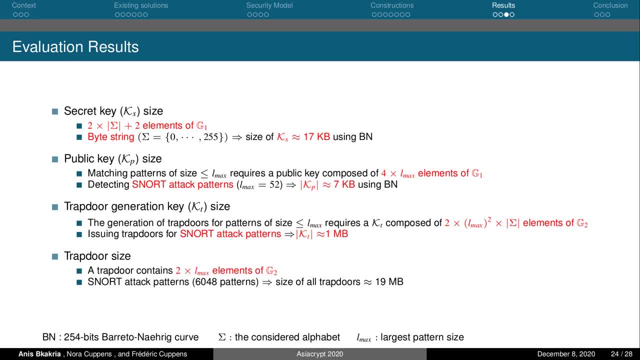 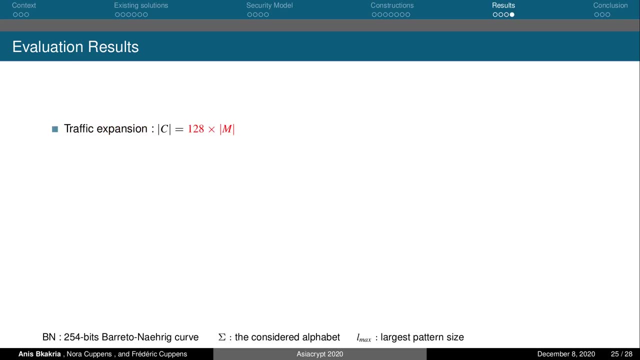 the size of the largest pattern and a secret key composed of two times the size of the largest pattern. Concretely, the total size of the trapdoors allowing to search all snort detection patterns is around 19 megabytes. Our constriction requires ciphertext that is 128 times the size of the plaintext. 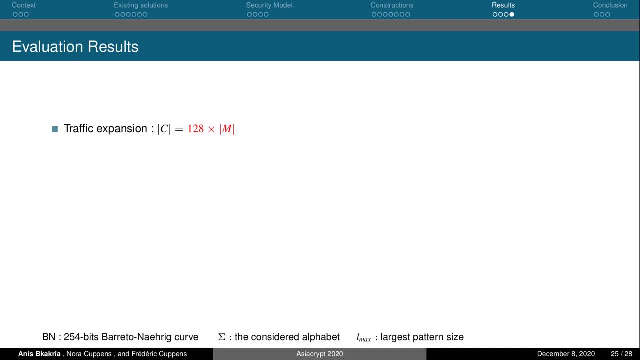 This is due mainly to the fact that we are encrypting each symbol of the plaintext separately. As for encryption complexity, the encryption of each symbol requires exponentiations in the group g1. concretely, our construction can achieve an encryption throughput of 25 kilobytes. for pattern detection, we are only able to achieve a throughput of 11 kilobytes per 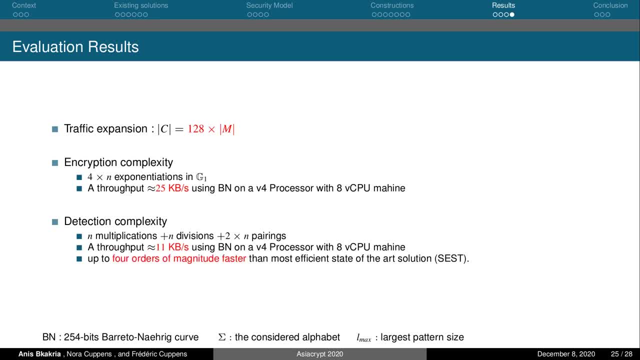 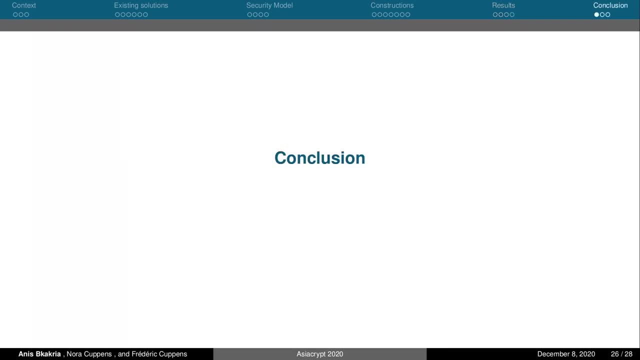 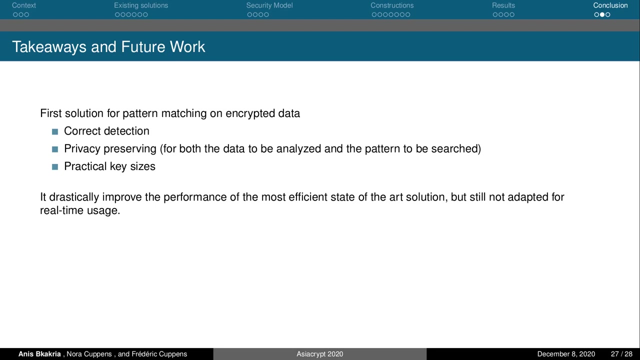 second. so despite this quite low detection throughput, our construction is up to four orders of magnitude faster than the most efficient state of our solution. okay, this brings me to the conclusion of this talk. so we propose the first solution for arbitrary pattern matching or encrypted data that provides correct detection and privacy protection for both. 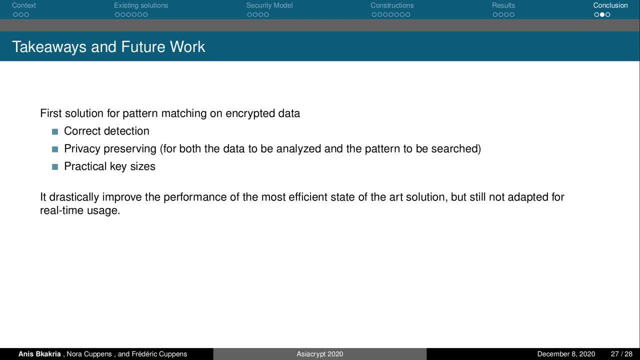 the encrypted data and the analysis patterns without requiring cryptographic keys with impractical sizes. our solution drastically improves the detection performance compared to similar existing approaches. you, however, the achieved performance are still not adapted for real-time usage. as a future work, we are working to enhance our construction to achieve better efficiency. 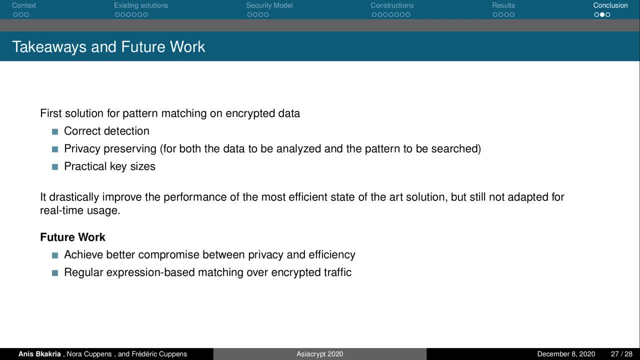 and to support regular express and search on encrypted data. thank you for your attention and i hope you enjoyed this talk.